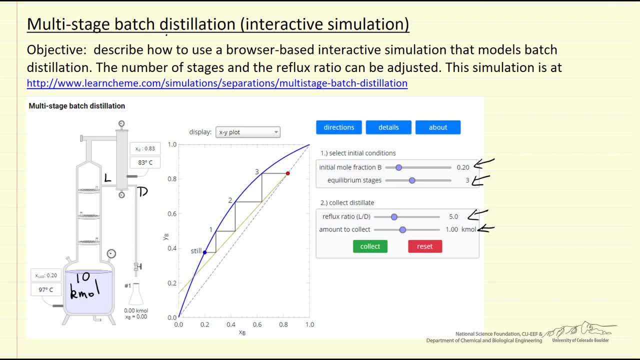 are continuously changing and we can see that in the simulation. So I'm showing an X versus Y plot here, where the still mole fraction- 0.2, is what we set at the start And you can see the distillate concentration is 0.83 at the beginning. 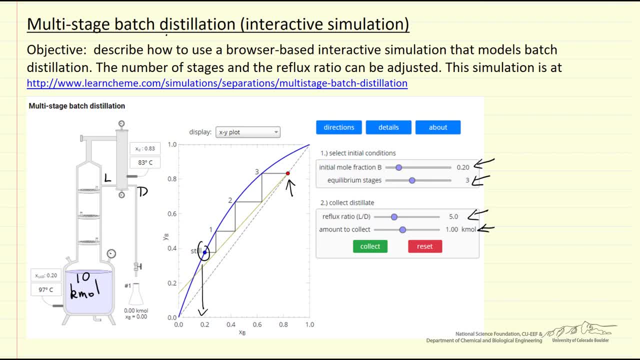 So we're getting significant separation, enhancement of the more volatile component. So let's look at the simulation and understand how things change as we change these variables. So here is the simulation and you notice the highest temperature is in the still 97,. 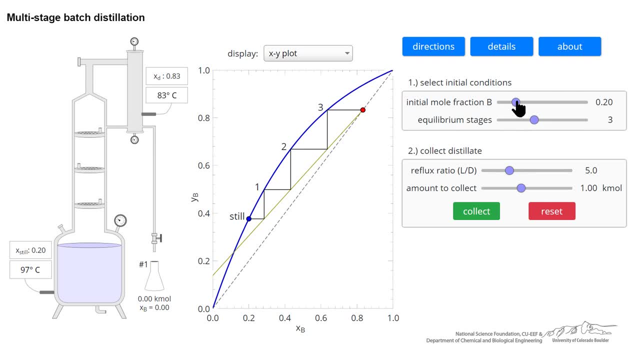 the lowest at the top. If I were to increase the mole fraction of B, the temperature drops. The reason for this is that we're increasing the amount of the more volatile component, the component with the lower saturation temperature. You notice how I move the mouse over this curve. it explains what it is, and likewise. 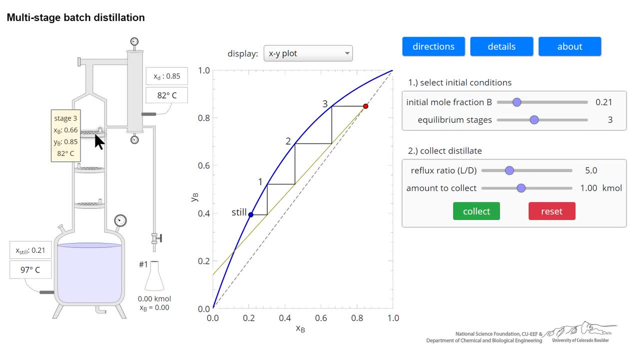 for the X equals Y curve. Likewise, if I move the mouse over a stage, then it shows the composition and the temperature of that stage. Now if I were to increase the number of equilibrium stages, then you'll notice that the mole fraction of the distillate goes up significantly. Now it's at 0.96.. Let me now dial that back. 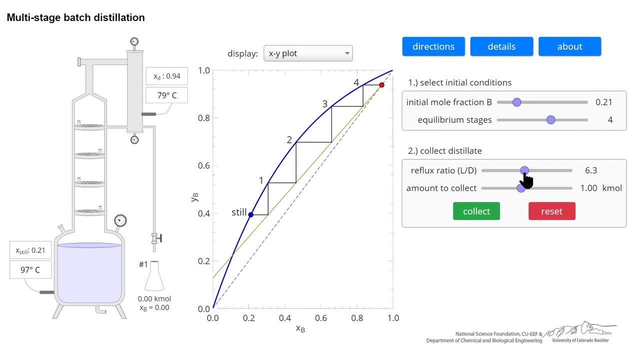 If I increase the reflux ratio we also increase the mole fraction of the distillate. So when I hit collect then you'll notice the mole fractions are decreasing, both the still and the distillate. This is a transient process And if I hit collect again, well, 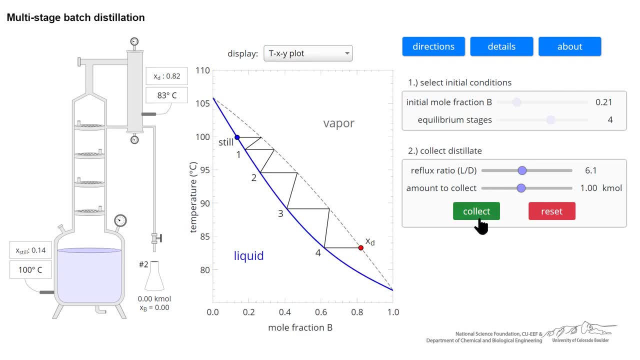 let me show you the behavior on the TXY diagram. If I hit collect, then notice the temperature is increasing and the mole fraction again. the distillate and still are decreasing. So after two samples the mole fraction in the still is down to 0.07.. The other display 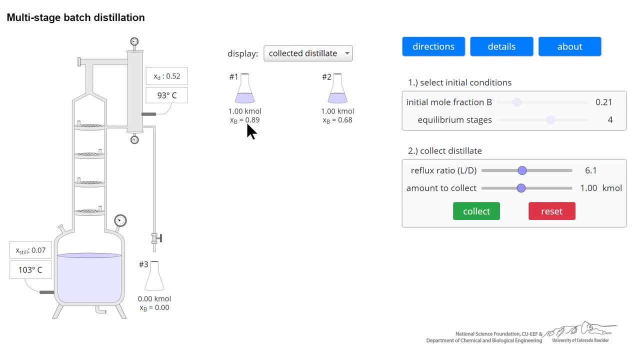 would be the distillate container. So the first one, mole fraction 0.89.. The second one, the mole fraction is only 0.68.. And if I continue collecting you'll see that this mole fraction now is significantly lower and we have very little of the more volatile component. 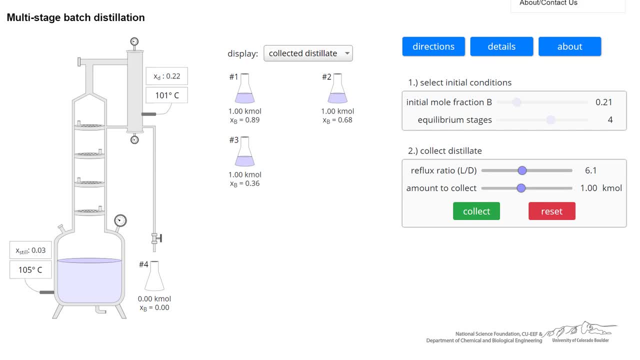 left in the still Temperature is up to 105 degrees. If I hit collect and go back to the beginning, I could collect a larger amount. I can change the reflux ratios, etc. Directions here have some of the same information that I explained. 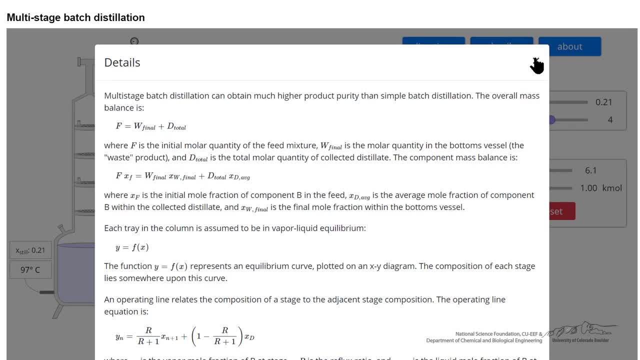 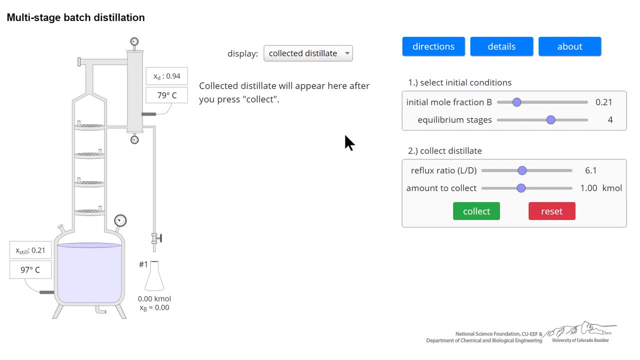 in this screencast And details show the mass balances used in the equations to determine these concentrations. So this equilibrium stage is multistage. batch distillation. 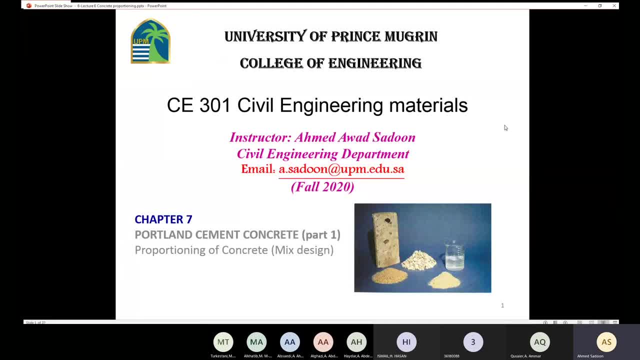 Let's get started. Today we are going to talk about the Portland cement concrete in Chapter 7.. In the previous lectures we learned about the ingredients of concrete. We explained the behavior of aggregates, whether it's fine aggregate or coarse aggregate. 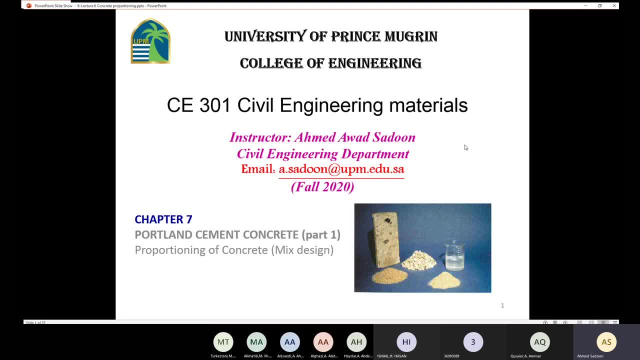 And also we talked about the cement- Portland cement- And also we talked about the water And finally, we talked about the admixtures. So now we have an idea about the ingredients of the concrete. So now we are ready in order to talk about the Portland cement concrete. 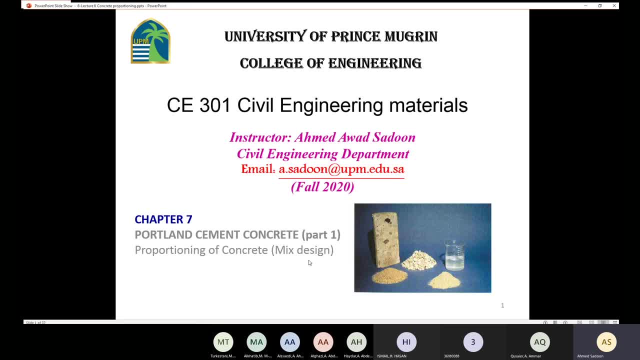 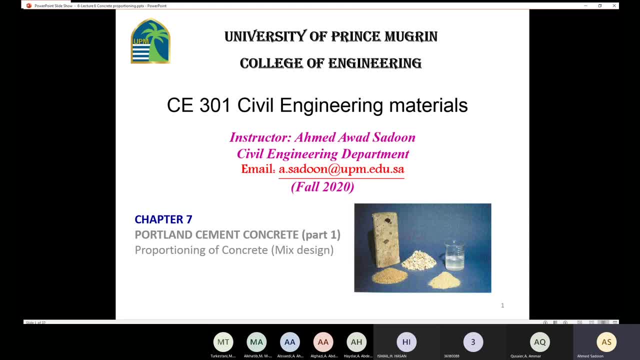 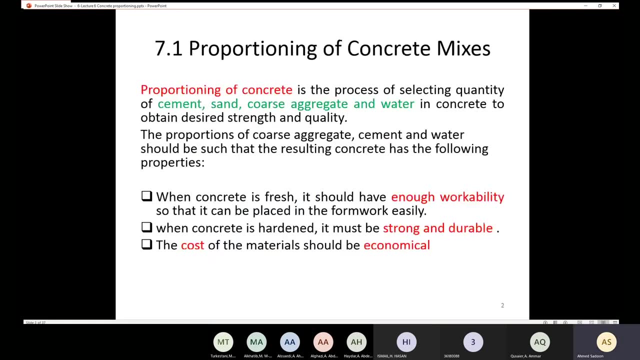 Which means that I need to know how much sand I need to put to the mix, How much gravel, how much cement, how much water and how much admixtures that need to be put in order to have good mix design. So proportioning of the concrete is a process of selecting quantity of cement, sand, coarse aggregate or the gravel and the water in the concrete. 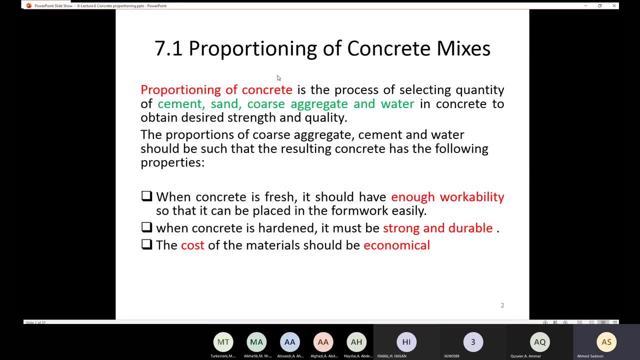 We are going to put all of this together in order to get concrete with desired strength and quality. So if I have a certain amount or quantity of cement, sand, gravel and the water, I will be able to target a certain strength and quality.